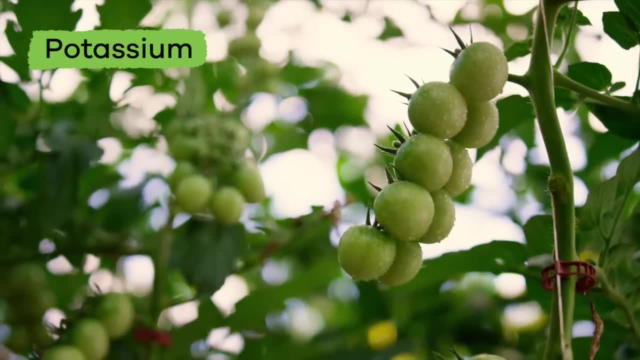 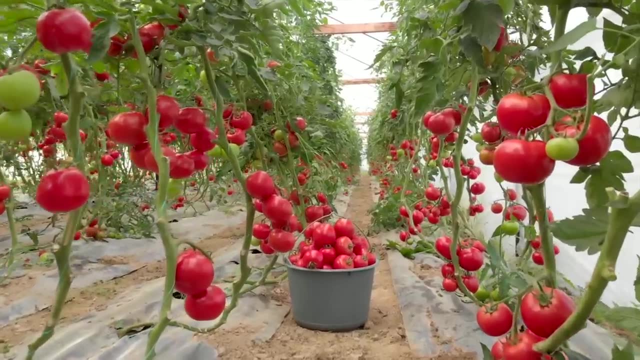 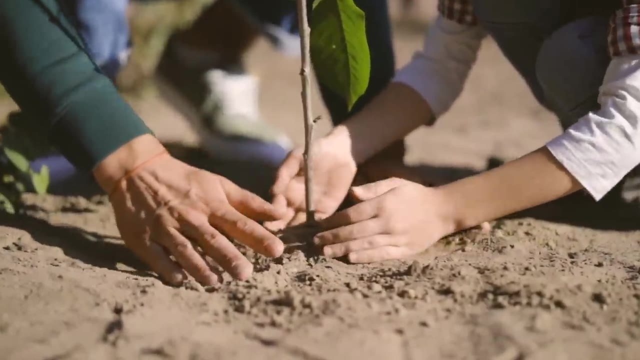 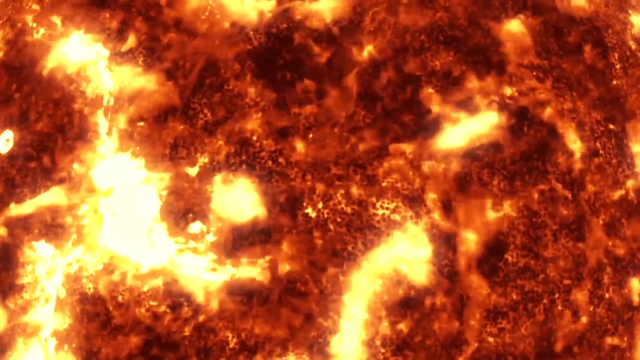 And potassium helps a plant fight off diseases. All of these nutrients help keep the soil healthy and create the perfect place for a plant to grow. Soil also gives support to plants and prevents them from falling over. Next up is sunlight. The sun is a super important part of plant growth. 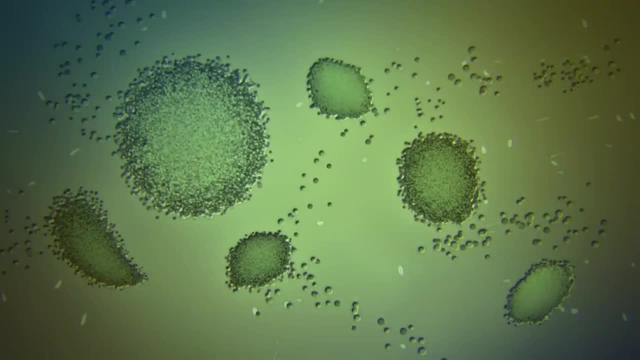 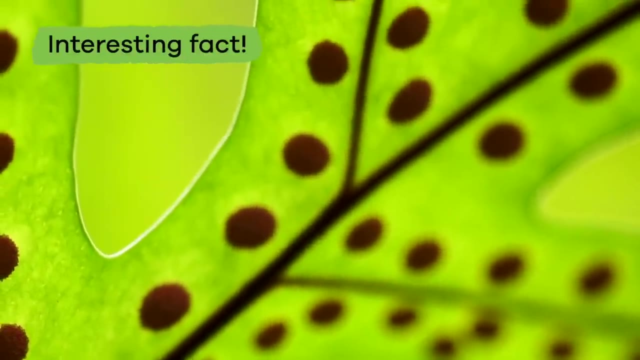 Plants use the energy from the sun to make their own food. Here is an interesting fact. This belong to the microbial verbe Reptiles. Flower plants love to eatantae, whichakapus- Alcohol really, So our plants choose to make it jackpot. 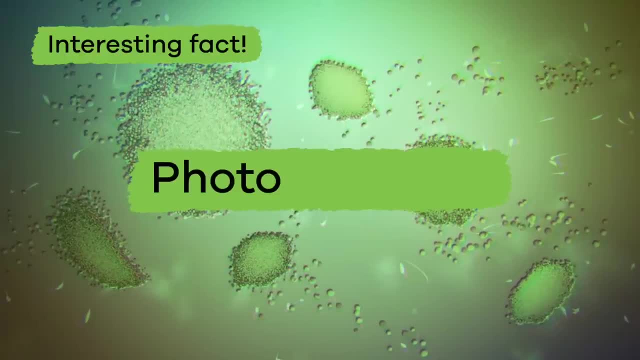 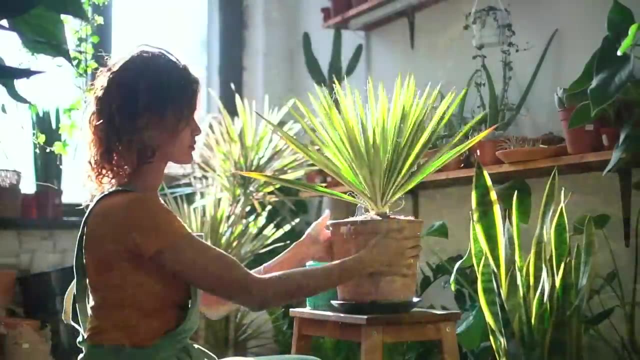 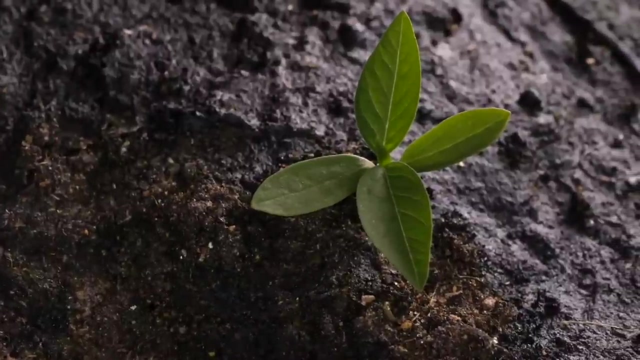 Say the next word: light. So humanificar is a process of barriers between light and light. Watch out the next word: Food making process is called photosynthesis. declarations, Video Talk about a big word. 野 Johann George. Even though sunlight is important, it also has to be the right amount. 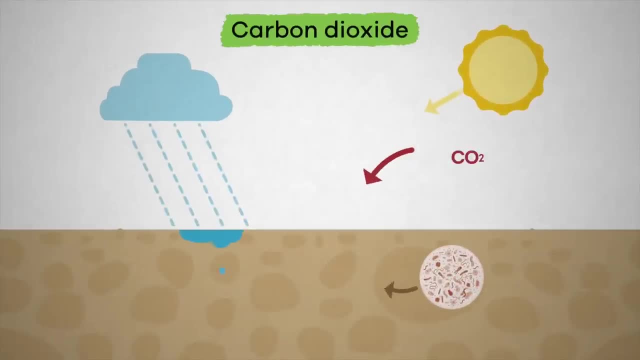 Vitamin C. Too much sun and a plant may whither Vitamin C. Time, temperature, Hydroxy Esther, Possibilities 수� beetonal oxidation Organ我說 lines Need兩 summoned with smallerammarizing CO2 from the air, which helps with photosynthesis. That means that the CO2 molecules 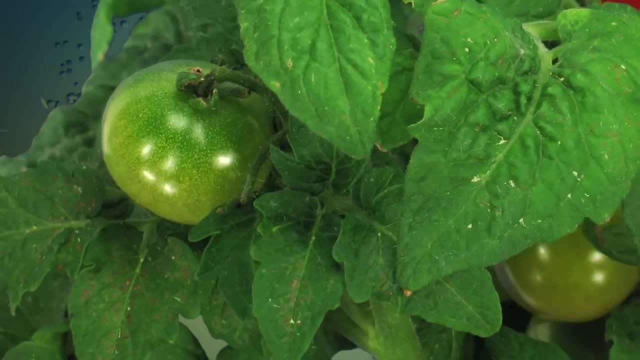 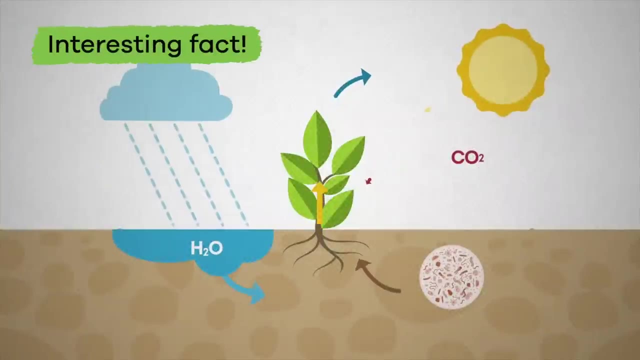 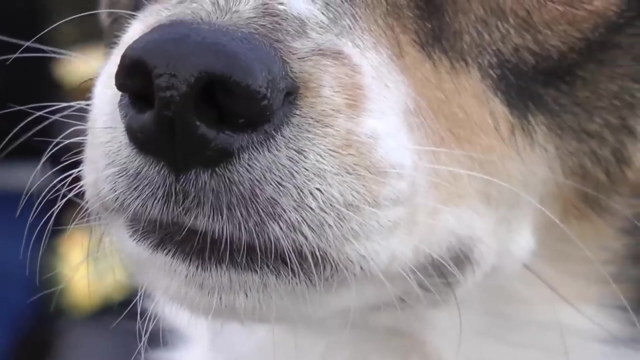 in the air, work with the sun to help plants make their own food, which in turn helps the plant to grow. Here is another interesting fact: During photosynthesis, plants release oxygen or O2, into the air. This oxygen is breathed in by animals, including humans like you. 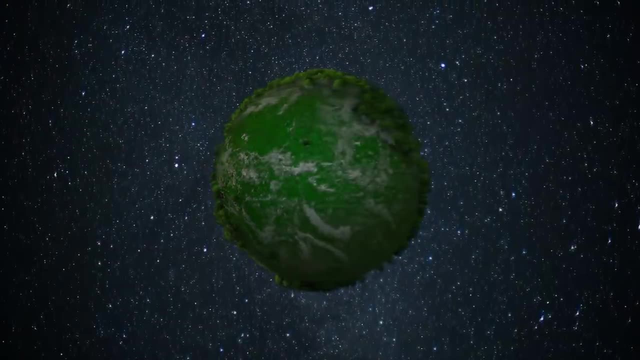 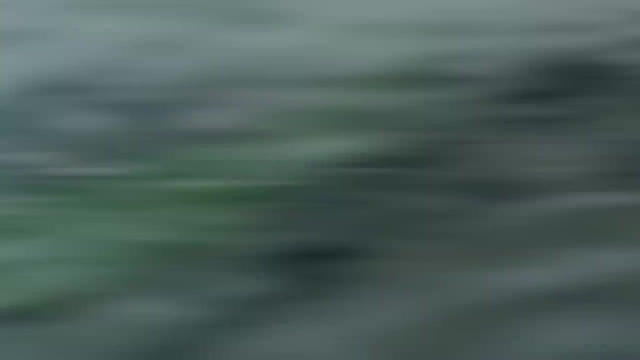 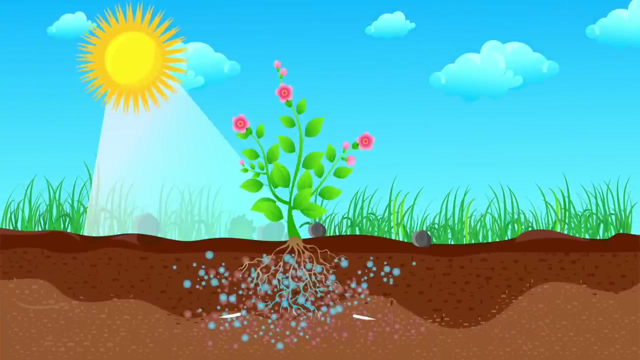 which is why plants are a vital part of keeping our planet healthy and alive. Last is our good old friend, water, which is also necessary to keep plants alive and help them to grow. The water a plant receives helps bring the nutrients found in the soil. 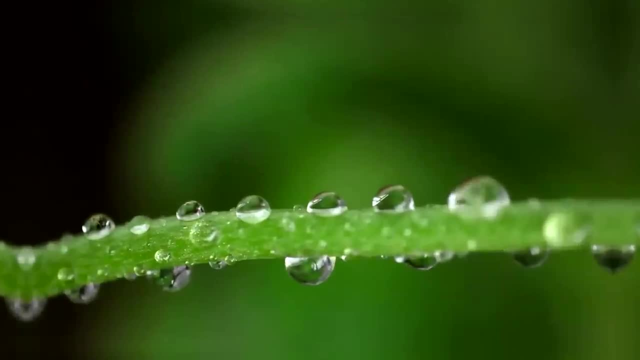 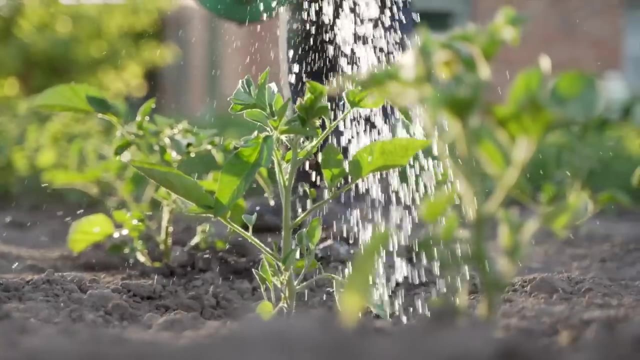 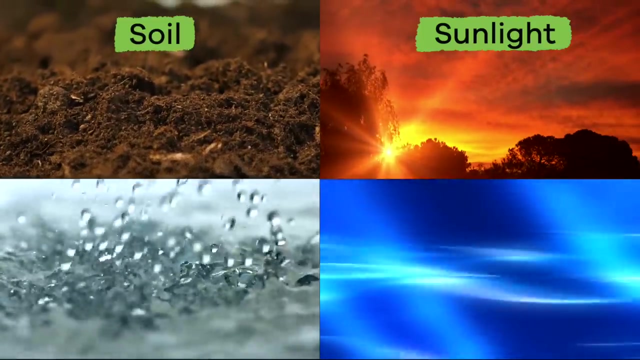 to the plant through their roots, stems and into their leaves. And, like sunlight, it is important for a plant to get just the right amount of water. It is pretty cool to see how soil, sunlight, air and water all work together to help plants grow. 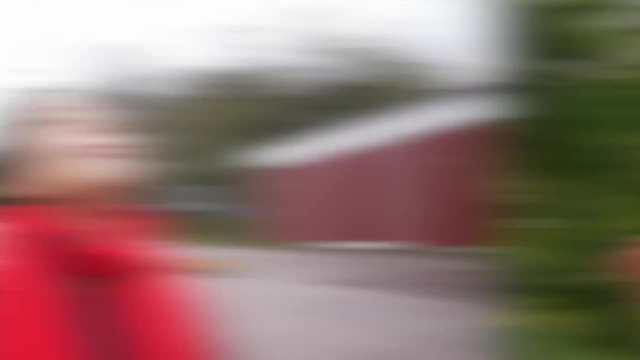 Were you surprised that plants need some of the same things that you need? It is pretty cool to compare and match these two things. If you want to know more about how plants grow, go to the link in the description below. If you want to know more about how plants grow, go to the link in the 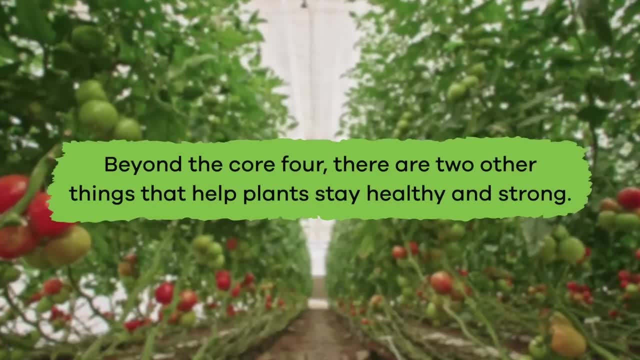 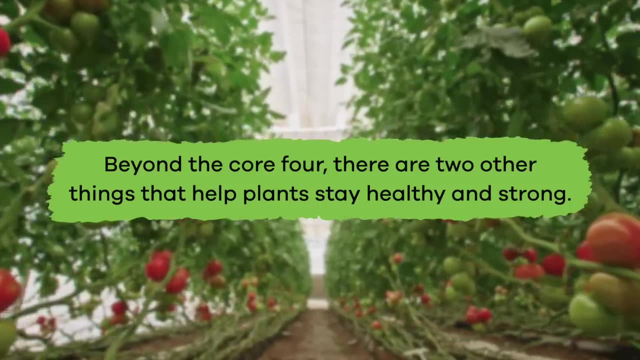 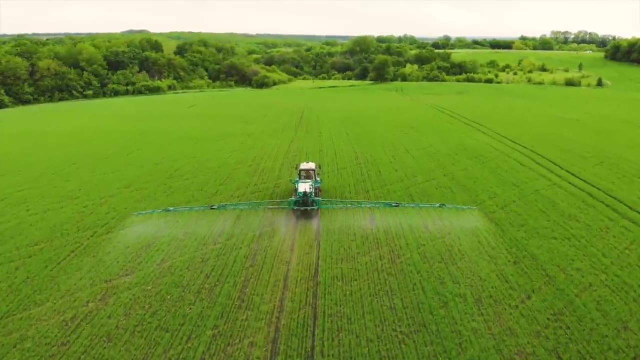 link in the description below. If you want to know more about how plants grow, go to the link in the description below. Beyond the core four, there are two other things that help plants stay healthy and strong. The first is temperature. Most plants grow well in warm daytime temperatures and cooler nighttime temperatures. 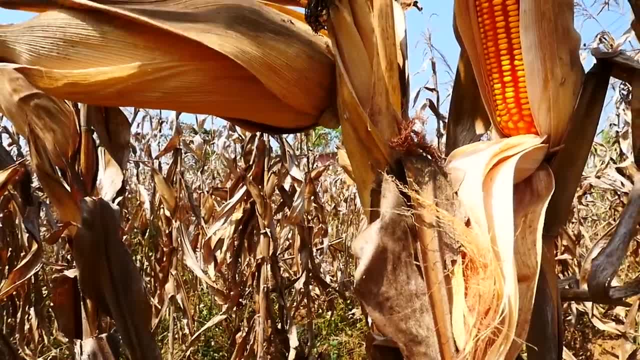 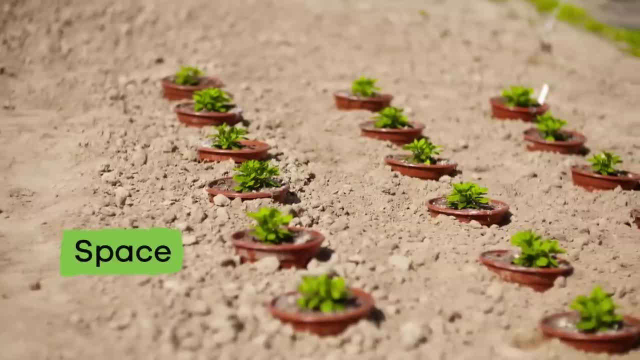 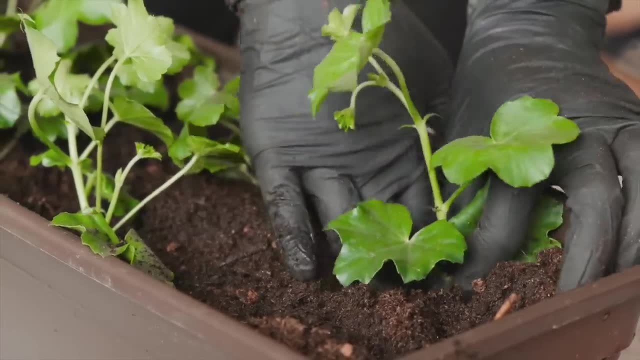 If it is too hot, plants will dry up and die. If it is too cold, they will freeze. Second is space. Plants need enough room to grow into their full size. Without this room, plants will not be able to develop deep enough roots to allow them to grow. 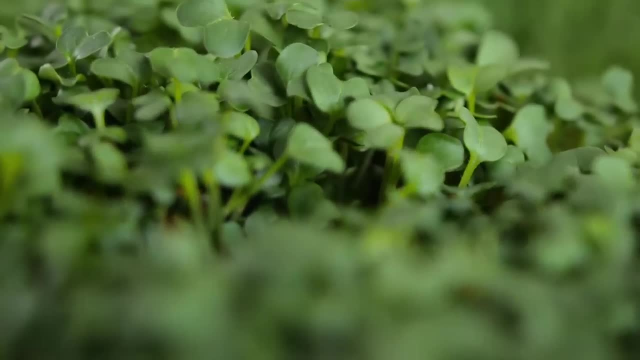 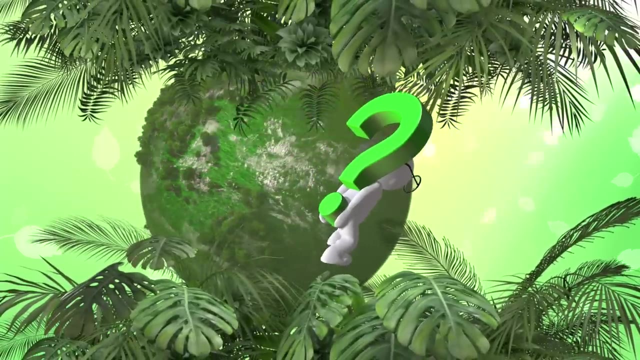 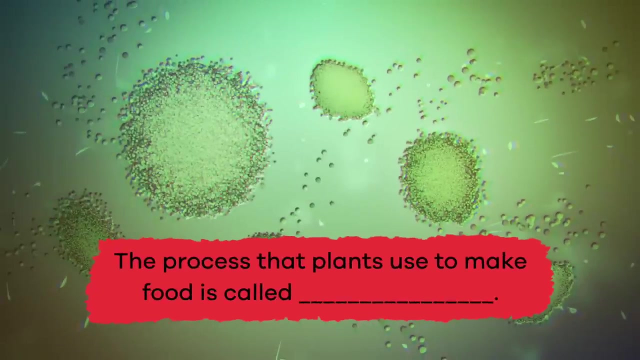 the way they are meant to, And if they are overcrowded, they might suffer from disease or not receive enough air. We have learned a lot about plants today. Are you ready to review? Let's get started. Let's do it. Fill in the blank. 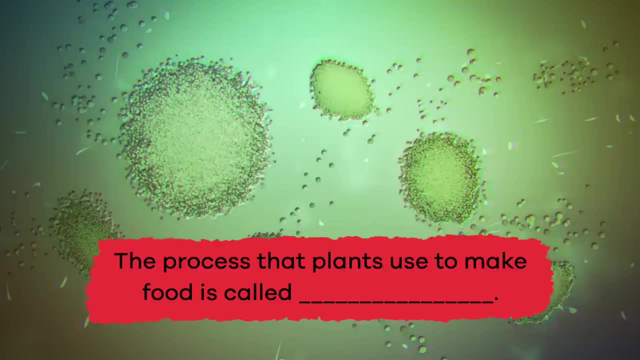 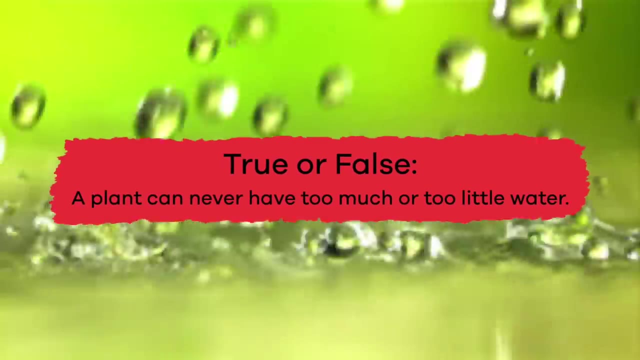 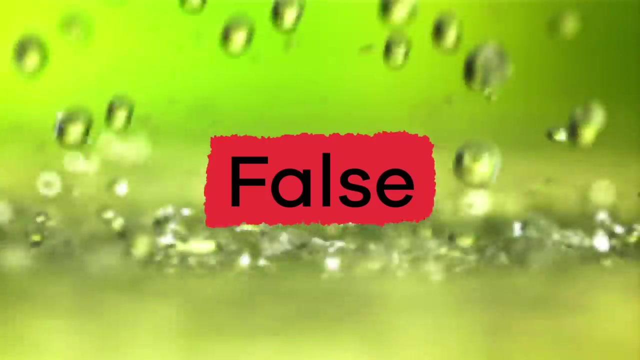 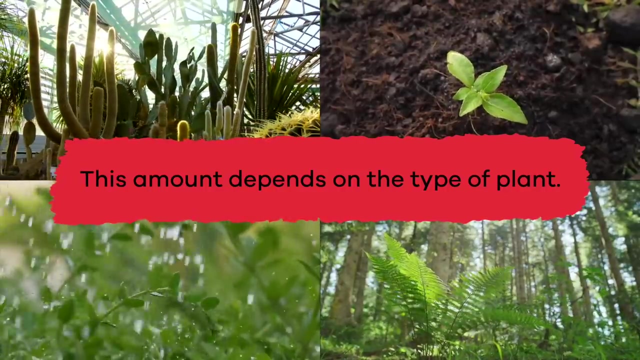 The process that plants use to make food is called blank Photosynthesis. True or false, A plant can never have too much or too little water. False Plants need just the right amount of water in order to stay healthy. This amount depends on the type of plant. 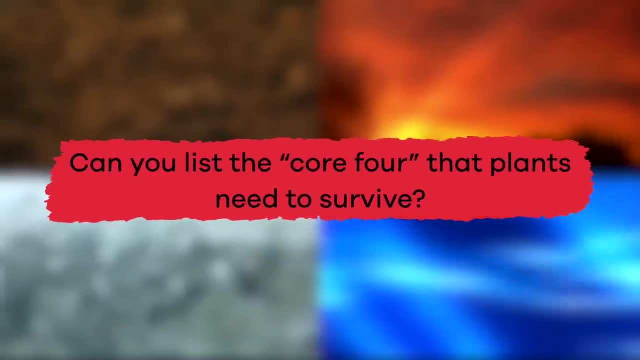 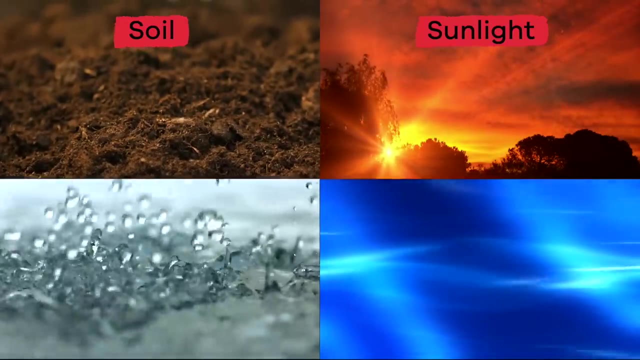 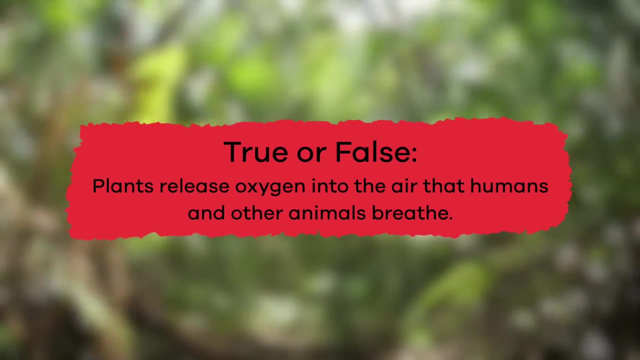 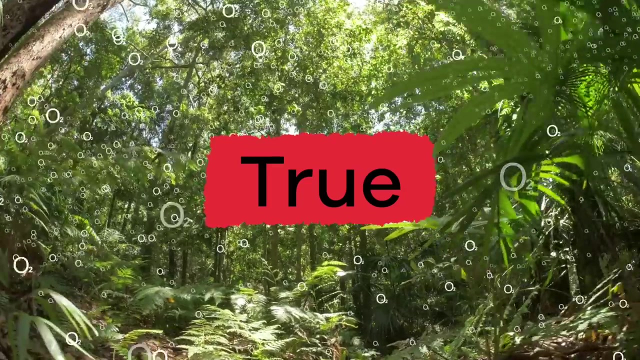 Can you list the core four that plants need to survive? Possible answers include soil, sunlight, air and water. True or false? Plants release oxygen into the air that humans and other animals breathe. True. Fantastic job, friends. False Plants release oxygen into the air that humans and other animals breathe. True. 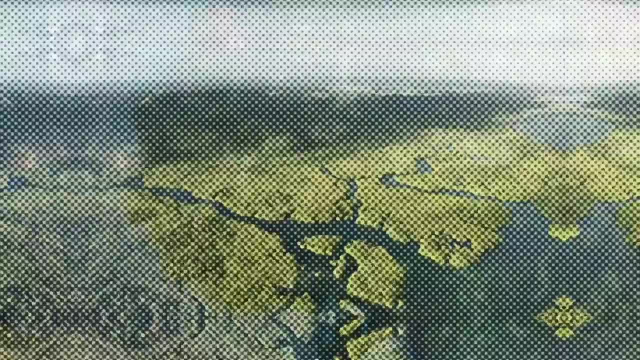 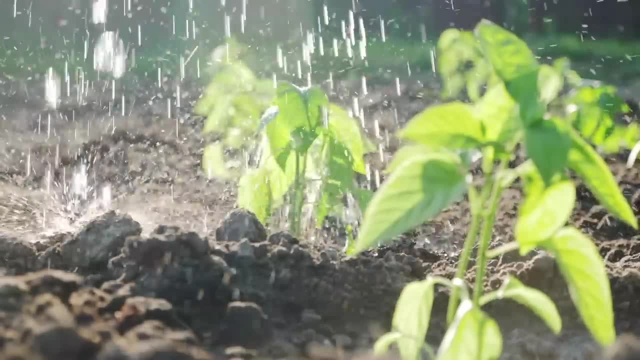 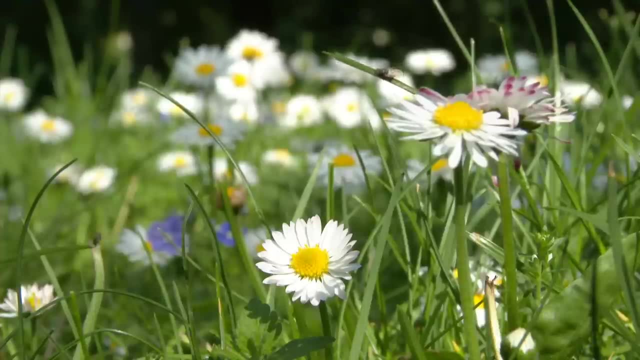 No matter where you live, plants are a necessary part of life on Earth And, just like people, plants need air and water to survive. Whether it is the tallest redwood tree or the smallest wildflower, plants are constantly growing and helping keep the environment healthy and safe.